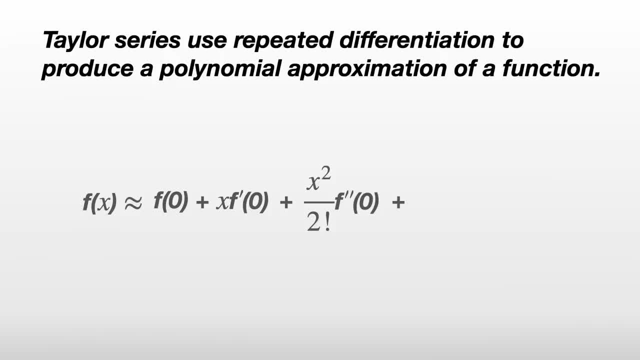 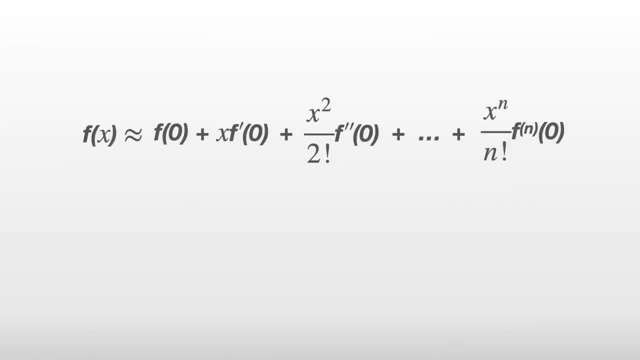 of 0 plus x, squared over 2 factorial times f prime, prime of 0, and so on, up to a term in x to the power n. For example, if f of x is equal to e to the minus x, then the Taylor series is 1 plus. 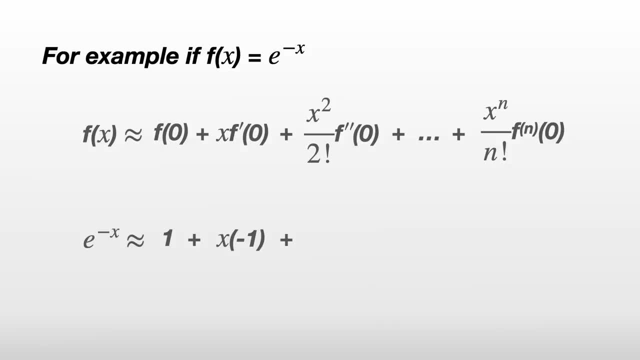 x times the derivative of e to the minus x at x equals 0, which is minus 1, and so on. The second order Taylor series includes terms up to x squared and is 1 minus x plus x squared over 2.. And we have this big O x cubed to say there's some error there, because we've 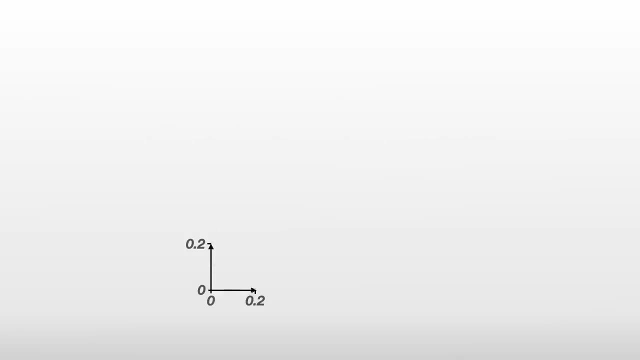 not included terms of x, cubed and above, And we can see that the Taylor series follows the original function quite well to begin with and then gets worse over time And it doesn't get better after that. For x bigger than 1, the Taylor series shoots up towards infinity as this x squared term begins to. 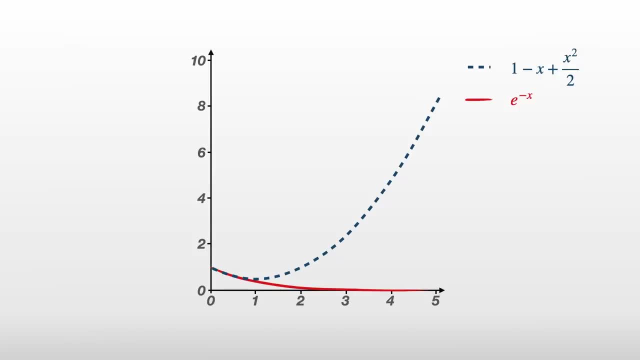 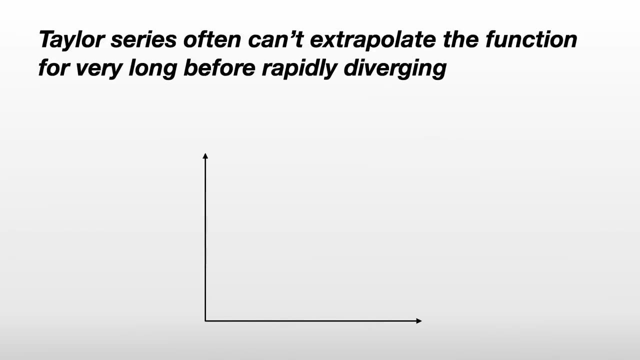 dominate Meanwhile. e to the minus x gets smaller and smaller with increasing x, And it's unfortunately a general property of Taylor series that they often can't extrapolate the function for very long Or rapidly diverging to positive or negative infinity. Pardee approximants often follow the function more closely. for longer We'll figure out. 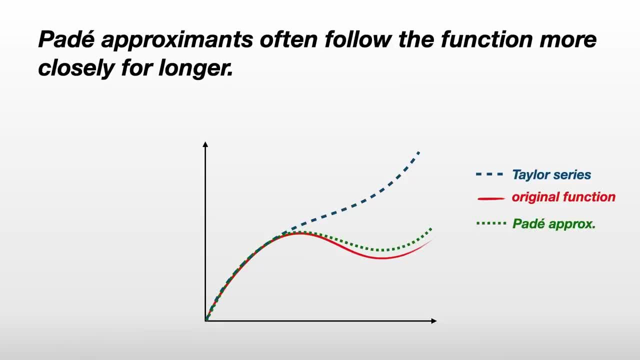 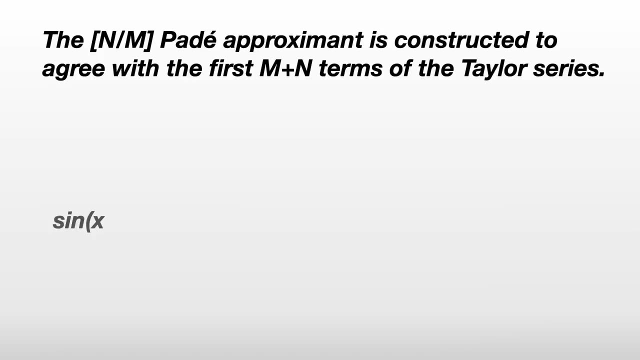 why. this is soon enough. but let's start by constructing one. The n over n Pardee approximant is constructed to agree with the first n plus n terms of a Taylor series. So if we want a 2 over 2 Pardee approximant for sine of x, that will. 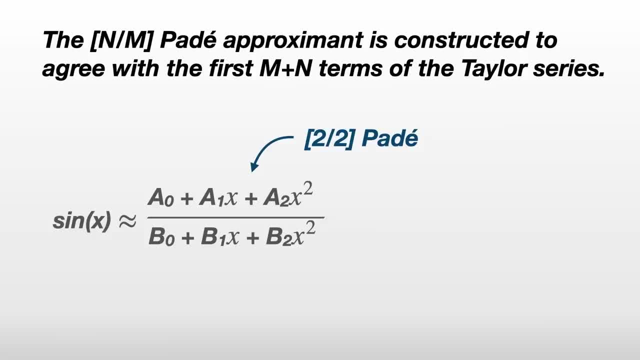 be in the form of a second order polynomial divided by another And, as I say, it needs to agree with the Taylor series of the original function up to n plus m terms. In this case, that's the fourth order Taylor series of sine of x. 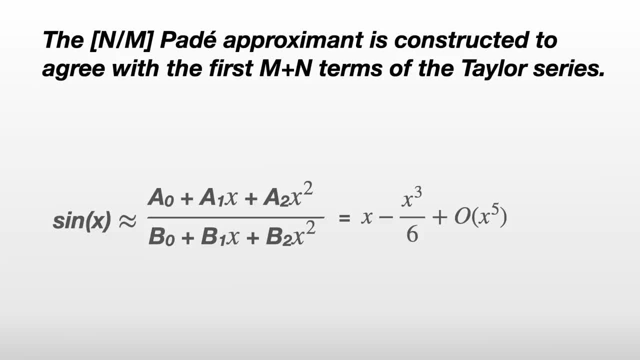 Now it just so happens that the x to the 4 term is 0, but that doesn't change anything, Notice. I've also included big O x to the power 5, just as a reminder that we can ignore any terms that pop up in the algebra larger than x to the power 4.. 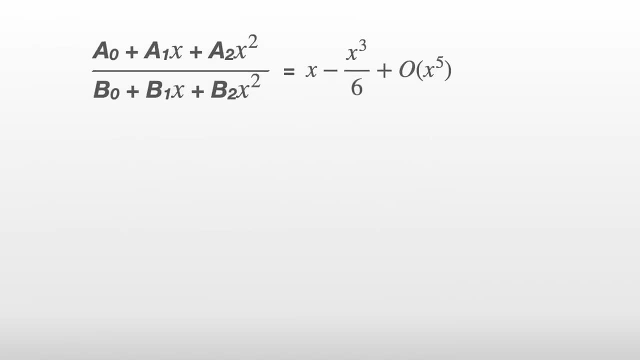 We equate the Pardee approximant with the Taylor series and the goal is to calculate the coefficients, the a's and b's of the Pardee approximant. Firstly, to make the algebra slightly easier, it's common to let b0 equals 1. This is without loss of generality, If you'd, 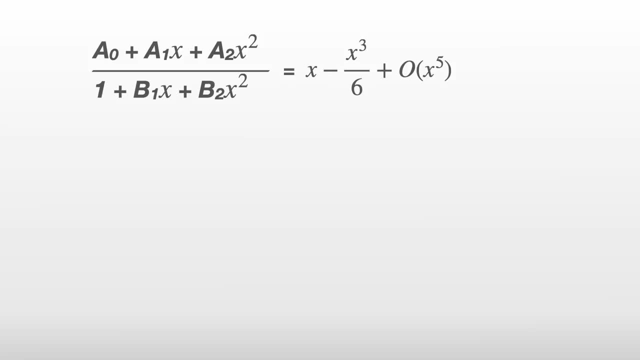 like to convince yourself that this is ok to do, start by dividing the numerator and denominator by b0, leaving the resulting 1 in the denominator and simply renaming the other coefficients back to 0. We can then bring the denominator over to the right hand side and multiply out the brackets. 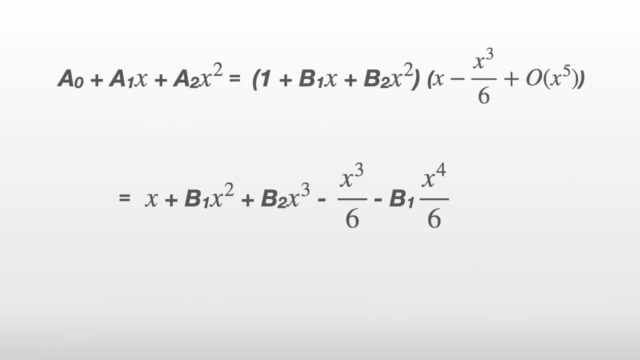 We can discard any terms larger than x to the power 4, or, more generally, we can ignore terms higher than the degree of the original Taylor series. Now we're left with one polynomial on the left hand side equals another on the right, So now we can solve a set of linear. 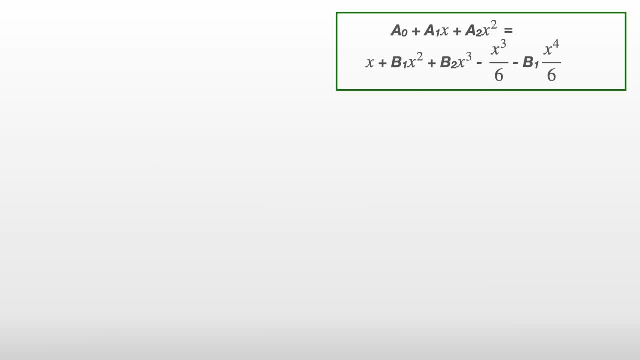 equations to make sure the terms in the like powers of x agree. We have the constant terms which give a0 equals 0, the order x terms which give a1 is equal to 1, terms in x squared which gives a2 equals b1, and now we've got two x to the power 3 terms and there aren't. 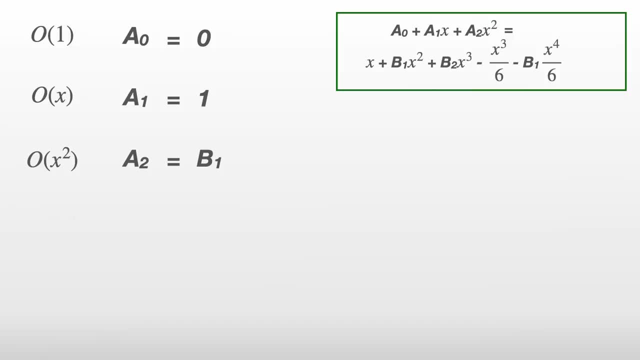 any on the left hand side. So that implies that the left hand side of this is 0 and that equals b2 minus 1 over 6, or b2 equals 1 sixth, The same with the x to the 4 terms We have. 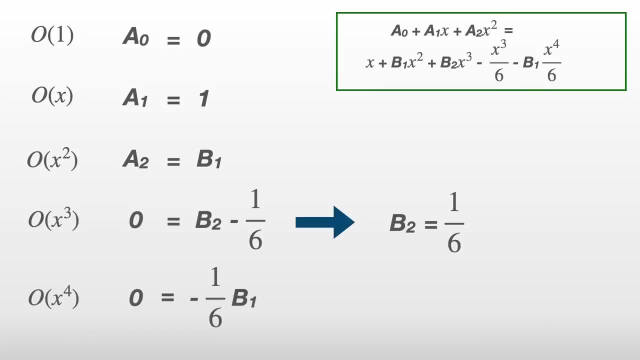 0 on the left hand side, and that equals minus 1 sixth of b1, which implies b sub 1 is equal to 0. And we already had a sub 2 equals b sub 1, so this must also be 0. We can then. 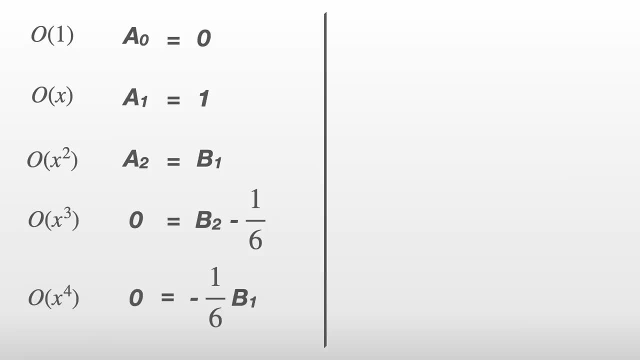 plug these coefficients back into the 2 over 2 part a approximant which gives x over 1 plus x squared over 6.. Now if we compare the function sine of x to our Taylor series and the part a approximants, 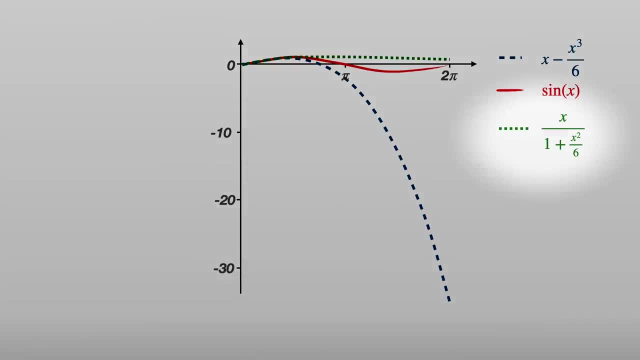 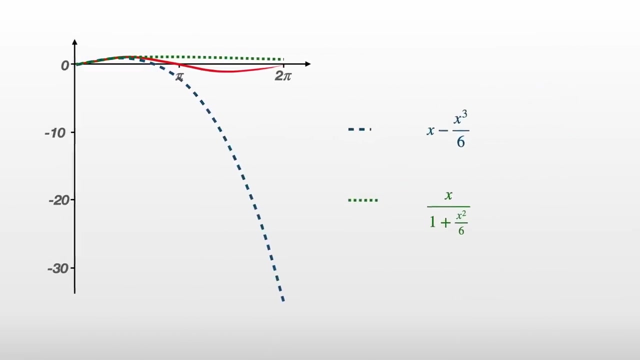 we can see that the part a approximant stays closer to sine of x for longer. At first this seems a bit like getting something for nothing. We have the same number of terms as the Taylor series in the part a approximant, so what is it that makes it better? Well, as x tends to infinity.